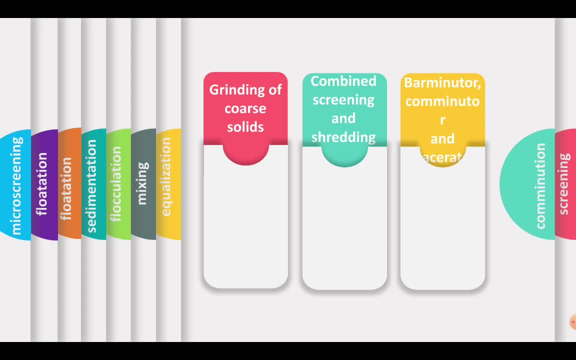 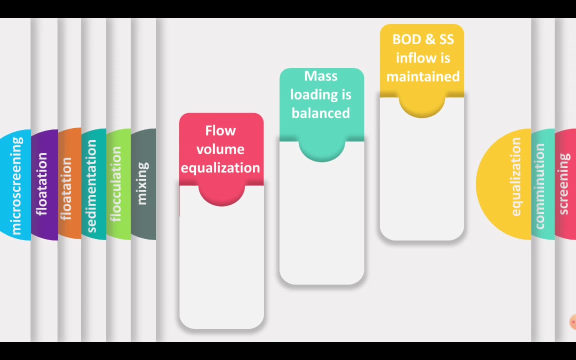 are there And macerators are there Which are used to conduct the process of comminution. Alright, Then we are going to see what equalization is. Now, see when we are saying equalization, it consists of three things. Okay, We are going to equalize the flow, Whatever the volume. 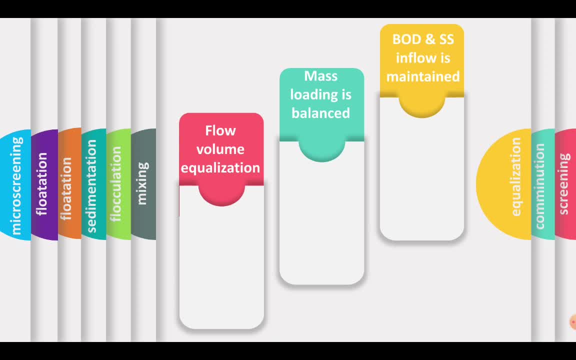 which will be incoming over the unit is equalized, then, whatever the mass, whatever the organic loading is there, Whatever the loading content of Westwater is there, it is balanced so that the unit will receive a constant concentration of Westwater, which is meant to be treated by it. Okay, 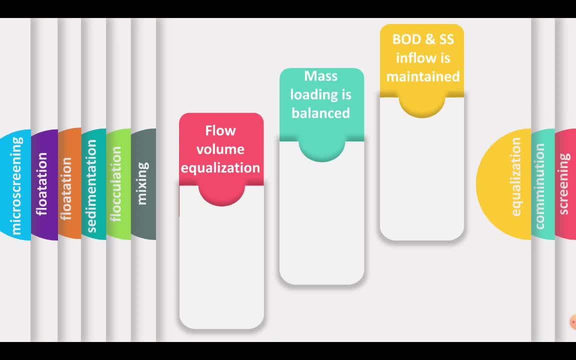 Then biological oxygen demand and suspended solid inflow is maintained. Okay, Whatever the units are there in Westwater treatment plant, they are supposed to act, they are supposed to have their maximum efficiency for a given concentration of Westwater. That's why this concentration is to be maintained, Okay. 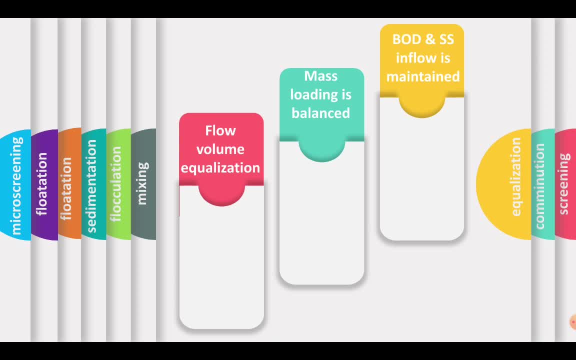 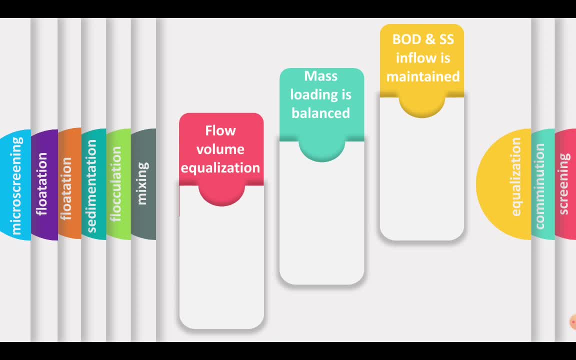 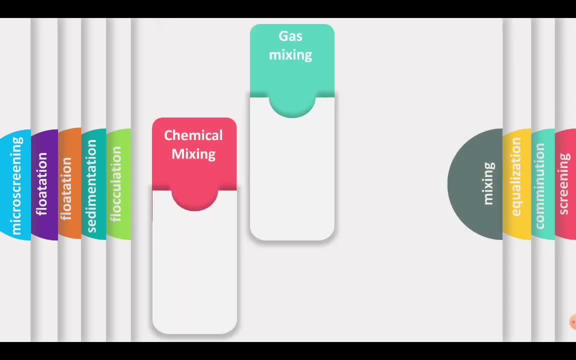 as equalization or simply flow equalization. Okay, Then we will see what mixing is. See, mixing is M. Mixing is targeted for the chemical, whatever the gases that we are going to introduce in order to support some process or in order to act as an active matter in the process. 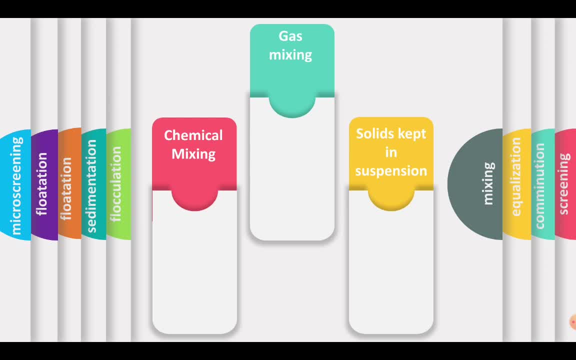 Okay, are to be mixed in during sludge treatment. chemical are to be mixed, then, while we are carrying out flotation. gas is to be mixed? okay. this is why mixing is also an another important process in wastewater treatment. okay, what we achieve by mixing? we keep the solids in suspension. 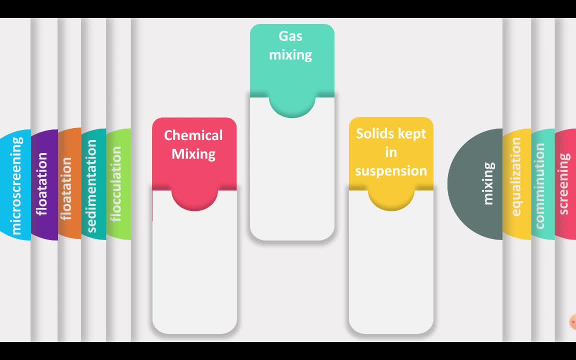 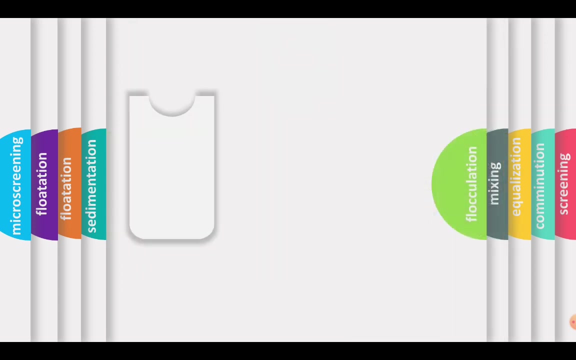 for example, while the flotation process, all the particles which are present inside the wastewater are kept in floating are kept afloat. they are kept in suspension by this mixing process when we are mixing the gas properly, when we are mixing air properly inside the unit. okay then what is flocculation? flocculation means formation of flock, see whenever wastewater is. 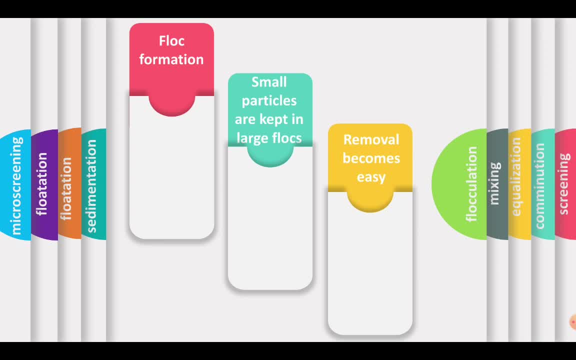 received. it contains small particles of wastewater, small particles of waste. now, these small particles do not settle easily, they cannot be removed easily. then what we can do over there is, we induce some chemical, we add some coagulant so that a flock cloud of small particle is formed which is easy to remove, which easily settles and thus can be taken care of by removal. 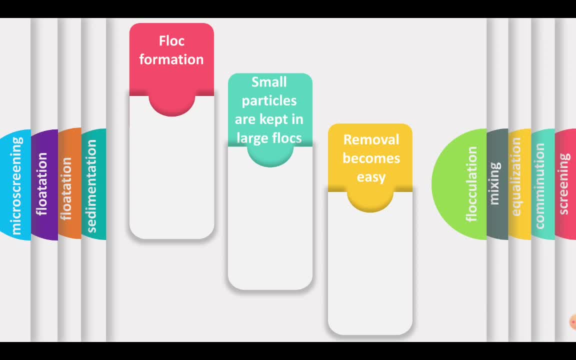 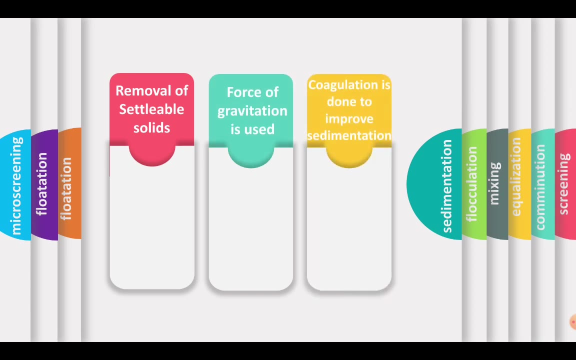 in, let's say, filtration, or in sedimentation tank. okay, this is why flocculation is another important process. okay, then we will see what sedimentation is. see sedimentation. the word sediment means particle. now, when we are saying, sedimentation is taking place in wastewater treatment. 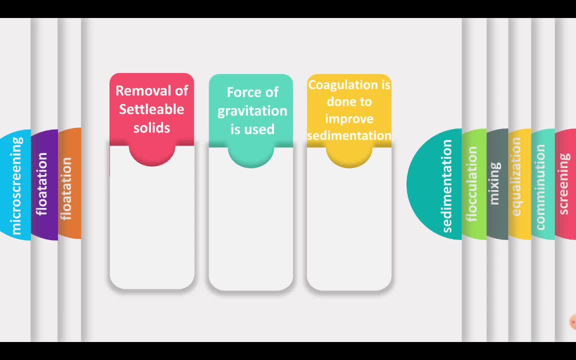 plant. we are looking at settling of particle. okay, which particle settleable solids- whatever the solids are there that can be settled by, merely by simply using the force of gravity- are removed in sedimentation tank. force of gravitation is used for this process now, in order to improve the sedimentation, in order to 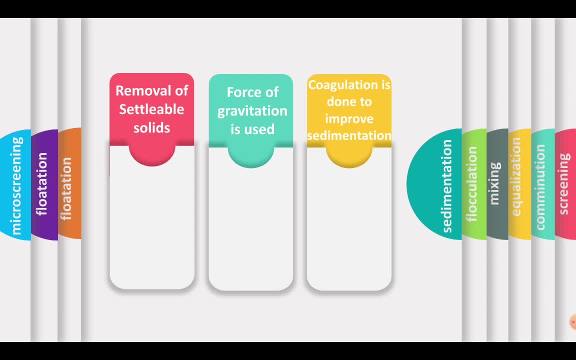 improve the sedimentation characteristics of the wastewater particle. what we do? we can add a coagulant to that. now we just saw coagulant. coagulant does what it adheres to the small particle. it forms a group, a cluster, a flock that is easily settable in wastewater. okay, 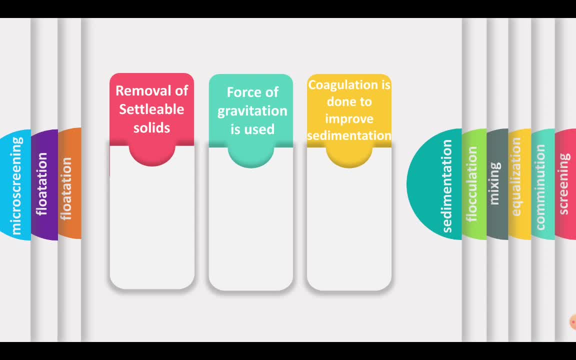 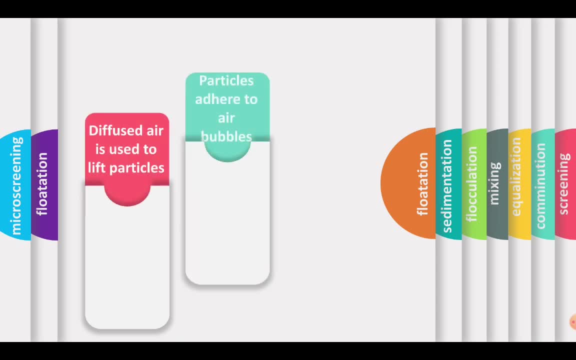 then this coagulation is done to improve, to aid the sedimentation process. okay, now let's see what flotation is. all right, flotation is done for getting rid of particle. okay now, which particle, the particle that have same specific gravity as that of water, can be taken care by the flotation process. now, 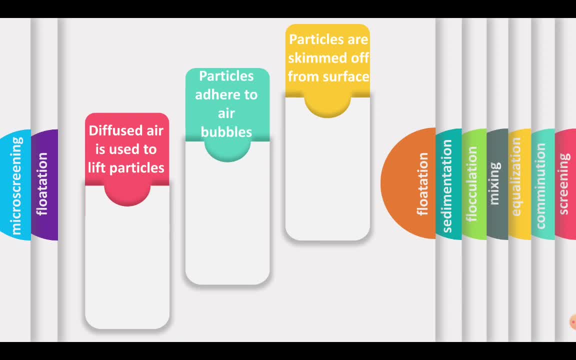 what we do in flotation. we inject with diffuse air in the west water in order to leave the particle. what happens over there is the air bubble acts as a defuse and flows with the air from the air bubble to the vessel to collect the particle, and it is then called as flotation. 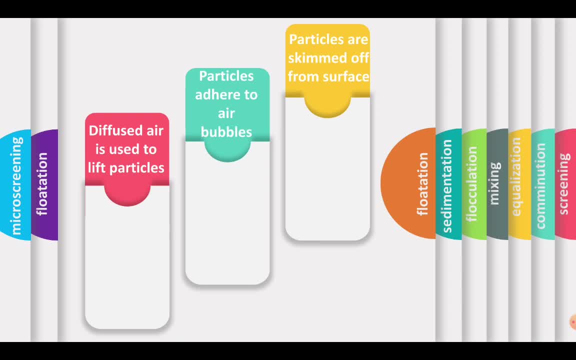 What happens over there is: the air bubble acts as a defuse and flows with the air to the particle, and since buoyancy of air bubble inside water is more, that's why it will go upward, and along with the upward motion it is going to carry some particles along with it. okay, now this. 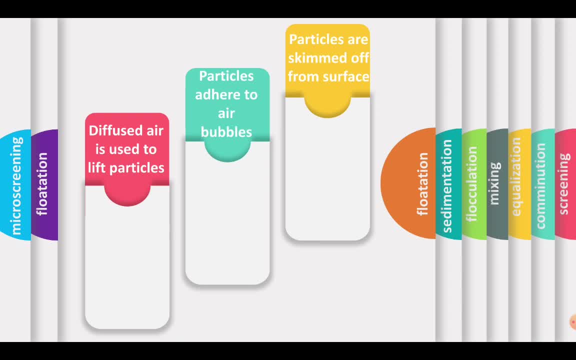 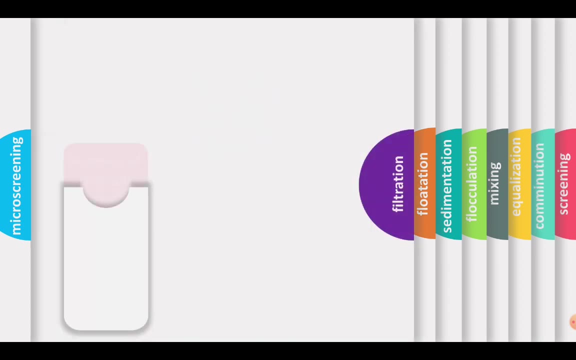 particle. when they come to the upper surface, to the topmost surface, they can be skimmed off, they can be removed, they can be directly chopped off from the upper volumes of wastewater. thus we can remove the non-settlable particles by using the process of flotation. okay, then filtration. what? 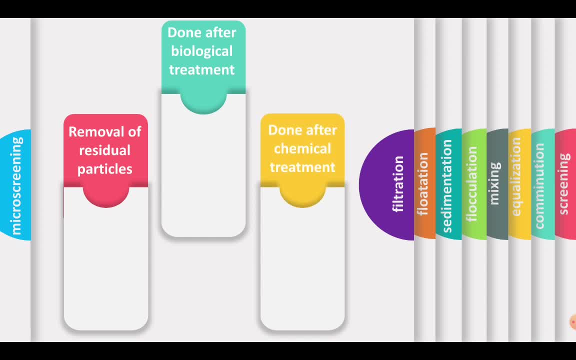 filtration is. filtration is nothing but removal of residual particle. whatever the flock that we have settled while we carried out sedimentation process, are removed in the process of filtration. okay, it is done after biological or chemical treatment. okay, chemical treatment, addition of chemical in order to receive some precipitated form of. 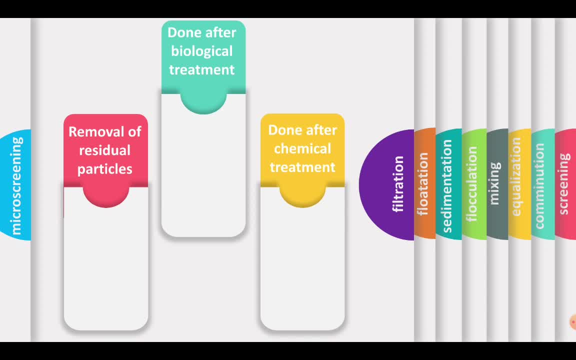 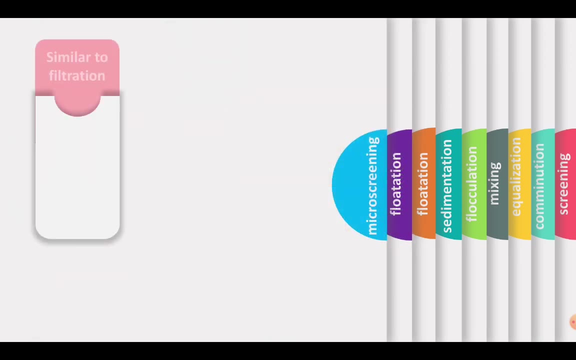 wastewater, organics or inorganic particle is done in chemical treatment and in biological treatment, whatever the biological action has taken and the particle which cannot be treated then biologically are then simply filtered out in filtration process. okay then micro screening. micro screening is very much similar to filtration. micro screening is utilized in order to remove algae from oxidation. 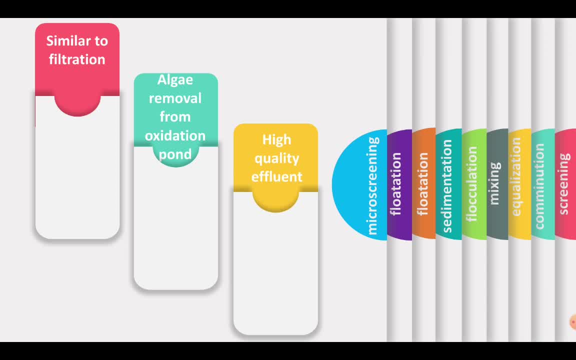 pond. when we are aiming at micro screening, we are looking at a very high quality effluent, because whatever the smallest size of particle is there can be removed by micro screening. which cannot be removed by filtration is removed by micro screening also. okay, so these were the physical unit operations or physical unit processes in wastewater treatment. 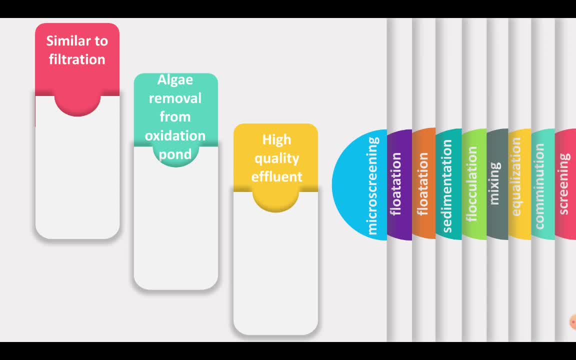 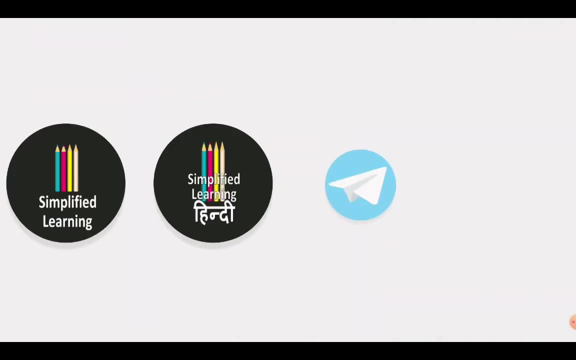 okay, we call them physical unit operation, because they follow the laws of physics and make the best physical forces without any involvement of biological or chemical action or process or concept. so that was all. do follow us on the main channel, which is simplified learning. if you are a hindi viewer, do check simplified learning hindi. follow us on telegram for quizzes, test series, notes, pdf, etc. and for the quirkiest meme of civil engineering, do follow us on instagram. till then, take care, bye, bye.